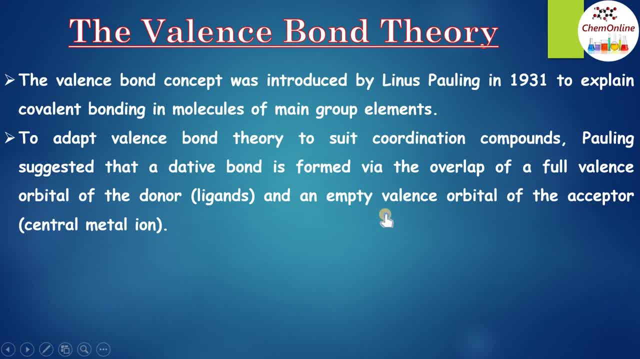 that is the ligand And an empty valence orbital of the acceptor atom, and usually the acceptor will be the central metal atom or central metal ion. So that is the central metal ion in the complex makes available an adequate number of empty orbitals for the formation of coordinate bonds. 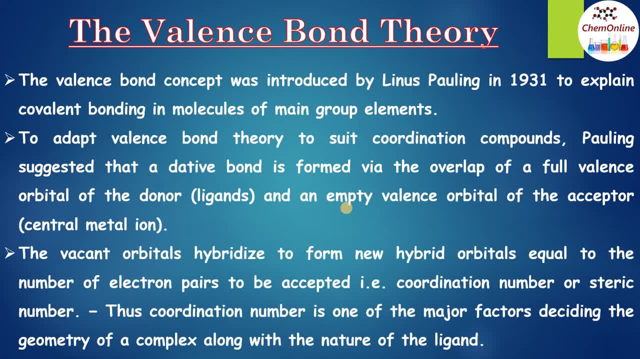 with suitable ligands. Now the vacant orbitals on the central metal atom or ion hybridize to form new hybrid orbitals, which is equal to the number of electron pairs to be accepted, which is known as the coordination number or steric number. So we can say that the coordination 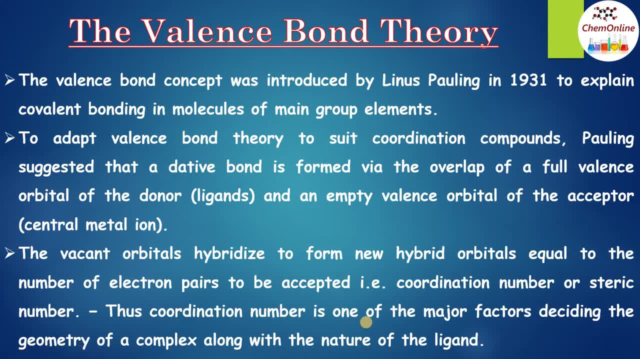 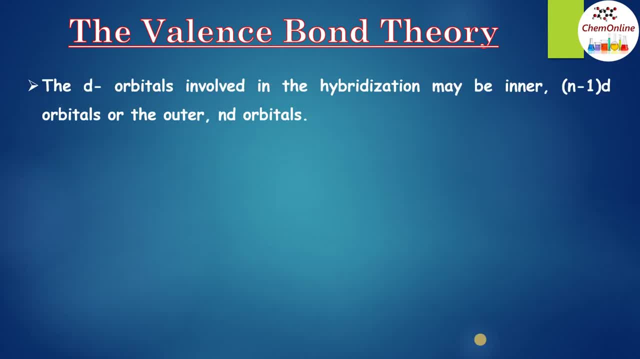 number is one of the major factors that decides the geometry of a complex, along with the nature of the ligand, Since the coordination compounds are usually formed by the transition and inner transition metal ions. generally, the d orbitals are involved in the hybridization And the metal d 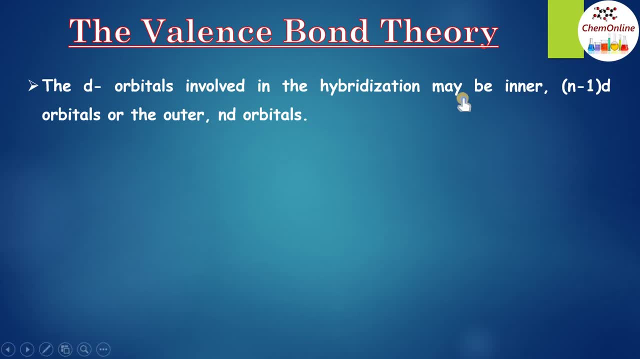 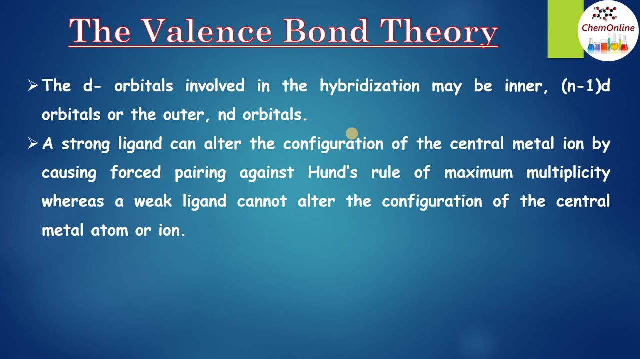 orbitals which involve in hybridization may be the inner d orbitals, that is, n minus 1 d orbitals, or it can also be the outer d orbitals, that is n d orbitals. The nature of the ligands will affect the final hybridization and geometry of the complex formed. A strong ligand can alter the configuration of the central metal ion. 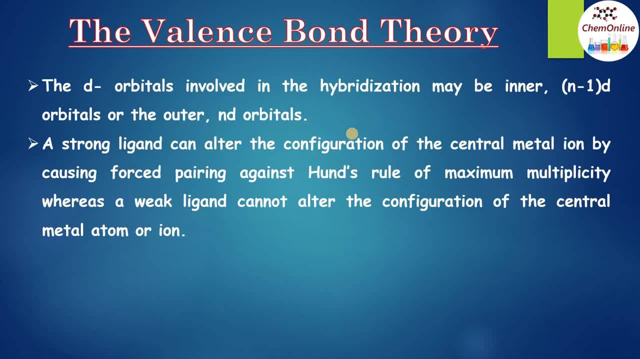 of the complex formed. a strong ligand can alter the configuration of the central metal metal ion by causing forced pairing against hans rule of maximum multiplicity, whereas a weak ligand cannot change the configuration of the central metal atom or ion. we will discuss about strong. 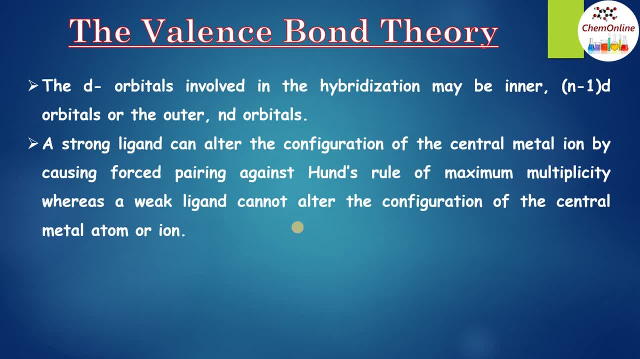 and weak ligands in the later examples. so in valence bond theory, the empty hybrid orbitals of the metal ion hybridize together and overlap with the fully filled orbitals of the ligand forming the ligand metal coordinate bone, and the number of such bones varies with the number of 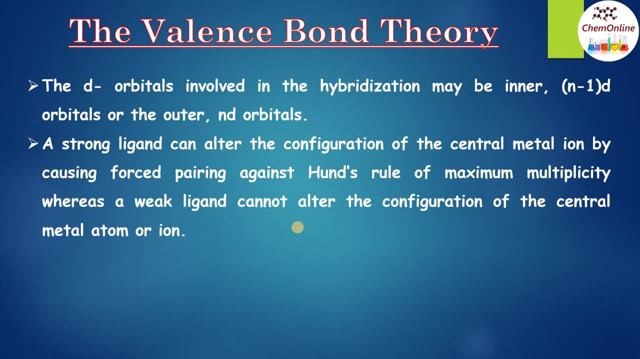 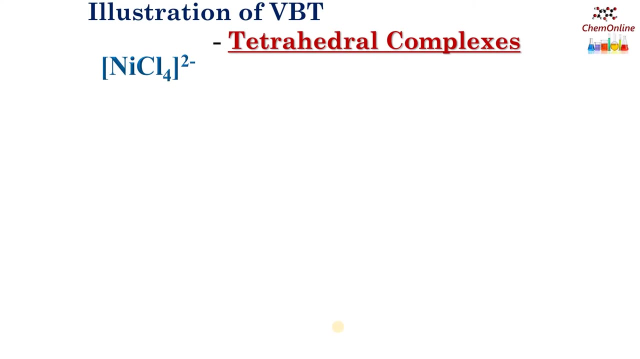 empty orbitals made available by the central ion. the valence bond theory has been able to account for many stereochemical and magnetic properties of coordination compounds. now let's see some examples of coordination compounds with different geometries, like tetrahedral, square planar and octahedral, and how valence bond theory, or vbt, is successful in explaining its structures. so first, 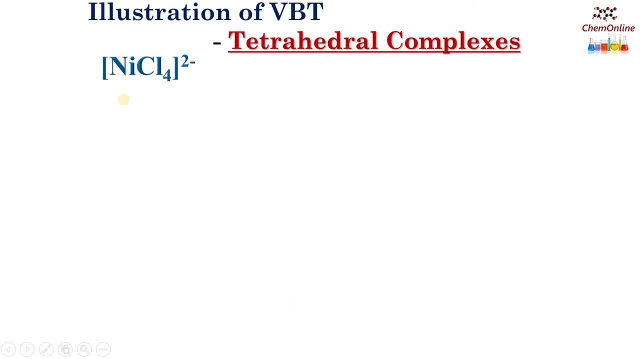 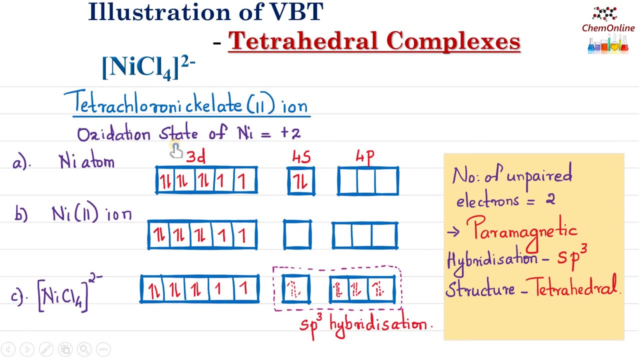 consider a tetrahedral complex, ni cl4 2 minus, tetra chloro nickelate 2 ion. so in ni cl4 2 minus we have to first determine the oxidation state of nickel. it is plus 2.. so first we have to write down the electronic configuration of the nickel atom. 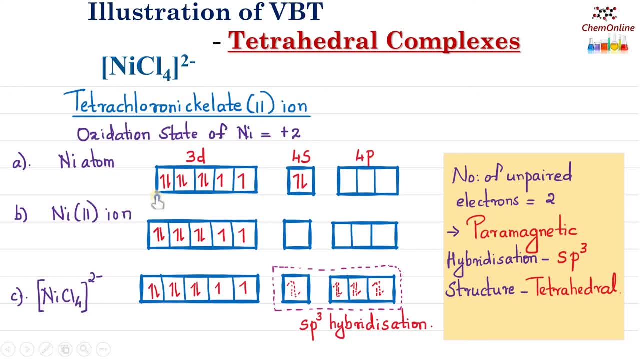 so nickel atom is a d8 species and it has the configuration 3d8 for s2 as it is shown here. now, in nickel 2 plus ion the two electrons are lost from the fours orbital first, so It will have a configuration 3d8- 4s0. 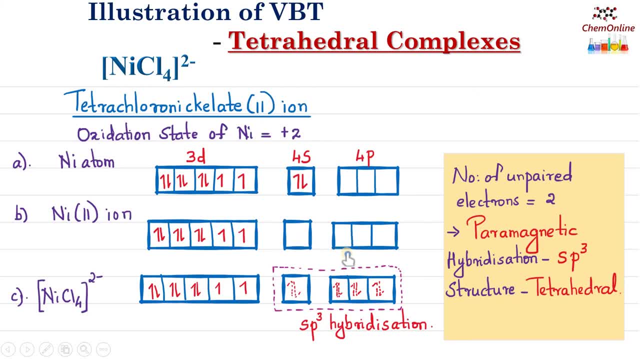 The outer 4p orbitals are also shown here. Now what happens when the 4 chloride ligands approaches the nickel 2 plus ion? The ligands will try to occupy the vacant orbitals in the metal atom. So here the vacant orbitals are the 4s and the 3 4p orbitals. 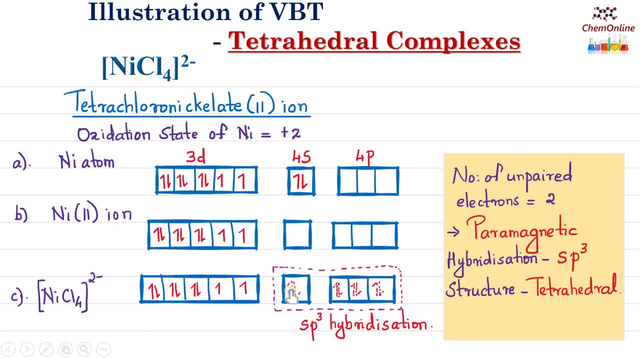 So these empty orbitals, that is, the 4s and 3 4p orbitals, will hybridize together to form 4 sp3 hybrid orbitals Which will be occupied by the electron pairs donated by the chloride ligand. The dotted arrows shows the electron pairs. 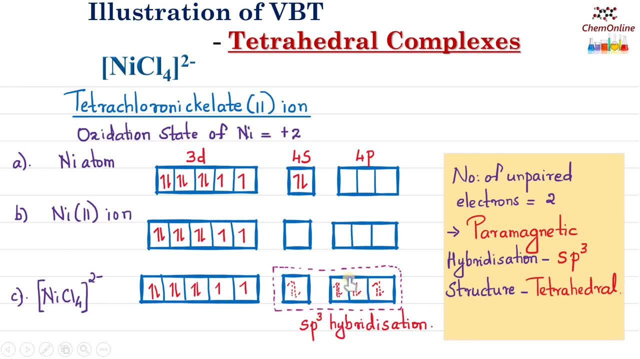 Donated by the chloride ligand. So in NiCl4 2 minus, the hybridization is sp3.. Since there are 4 sp3 hybrid orbitals, They will be oriented towards the corners of a tetrahedron, So the geometry of the complex or the structure of the complex will be tetrahedral. 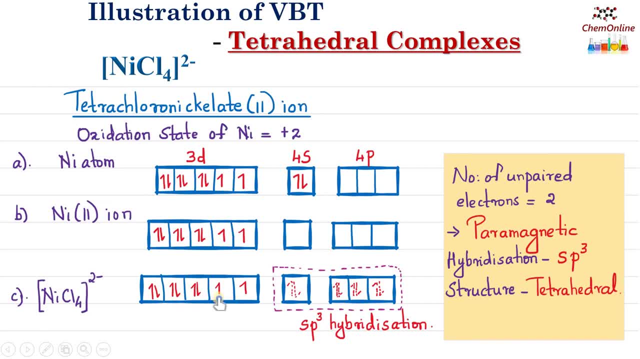 And you can see here in 3d orbitals There are 2 unpaired electrons And therefore The complex will be paramagnetic. So using VBT You can explain whether a complex will be paramagnetic or diamagnetic If there are unpaired electrons. 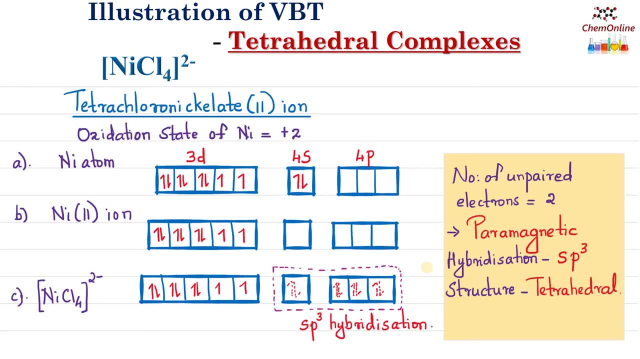 It will be paramagnetic, And if there are no unpaired electrons It will be diamagnetic. You can also explain the hybridization And from the hybridization You can predict the structure of the complex. So in NiCl4, 2 minus. 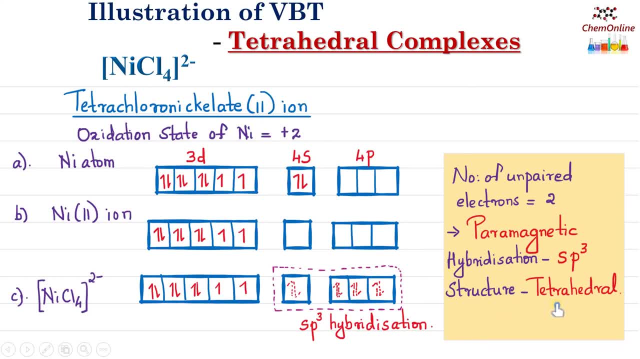 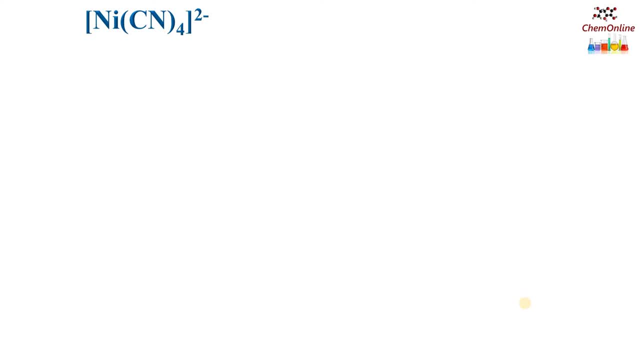 The hybridization involved is sp3. The structure is tetrahedral And the complex is paramagnetic. Now consider another complex of nickel: NiCl4 2 minus Tetra sino nickelate ion. Here also the number of ligands is 4.. 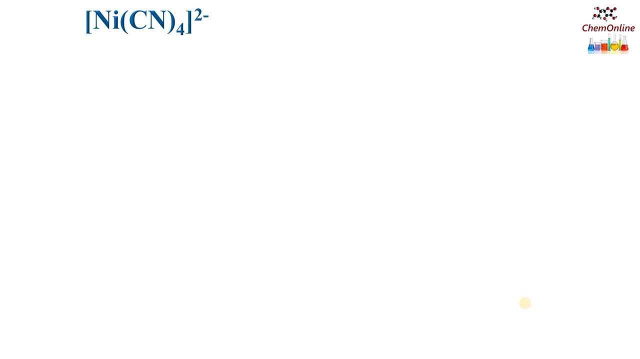 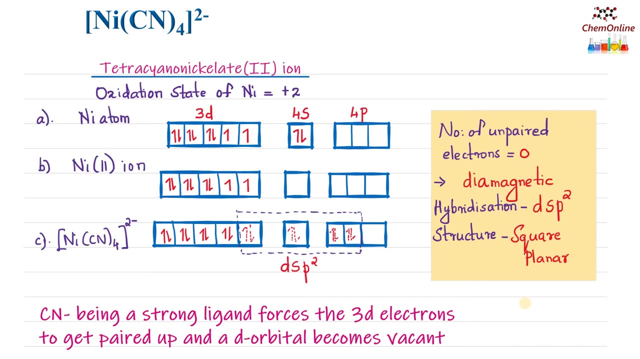 So the expected structure of the complex is tetrahedral. So let's see how VBT explains the Structure of NiCl4, 2 minus. So here also, the oxidation state of nickel is 2+, So nickel atom has 3d8, 4s2.. Nickel 2 plus ion. 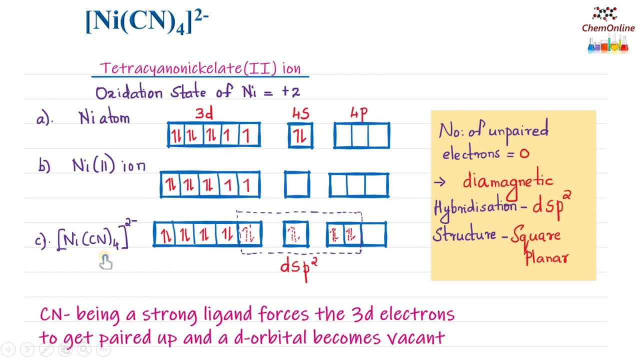 has 3d8- 4s0.. Now, when the 4 cyanide ligand approaches the nickel 2 plus ion- you can see here there occurs a pairing of the electrons. Cyanide ion is a strong ligand and it forces. 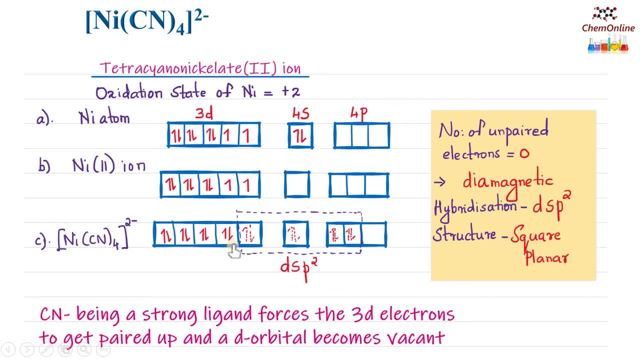 the 3d electrons to get paired up and a d orbital becomes vacant. So one vacant 3d orbital, one 4s and two 4p orbitals will hybridize together to form four dsp2 hybrid orbitals. So, contrary to NiCl4 2-, which involves an sp3 hybridization, here the hybridization is: 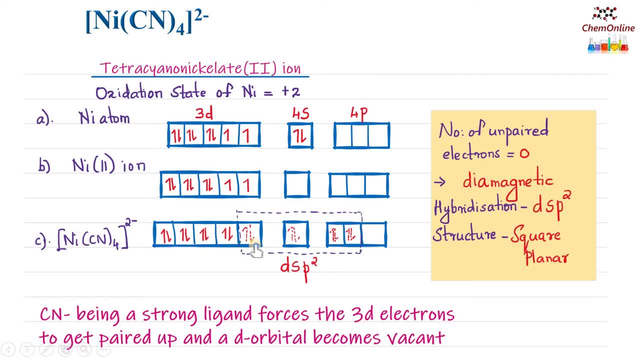 dsp2.. So when the hybridization is dsp2, the structure of the complex becomes square planar And in this case the number of unpaired electrons is 0.. You can see that all the electrons are paired up. So when all the electrons are paired up, the complex will be diamagnetic. according to VBD. 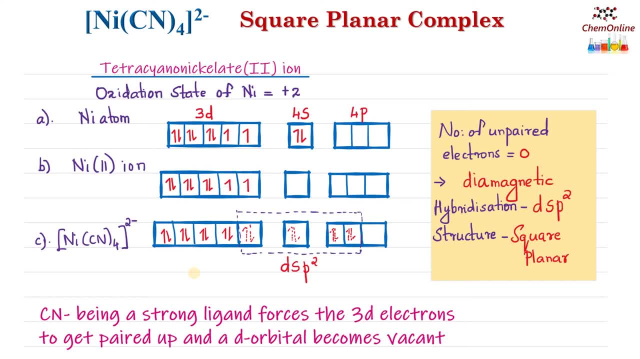 So in NiCl4, 2 minus, the cyanide ion is a strong ligand and hence it forces the electrons in the 3d orbital to get paired up, and the structure becomes square planar instead of tetrahedral, and the hybridization is dsp2.. And since all the electrons are paired up, the complex is diamagnetic. 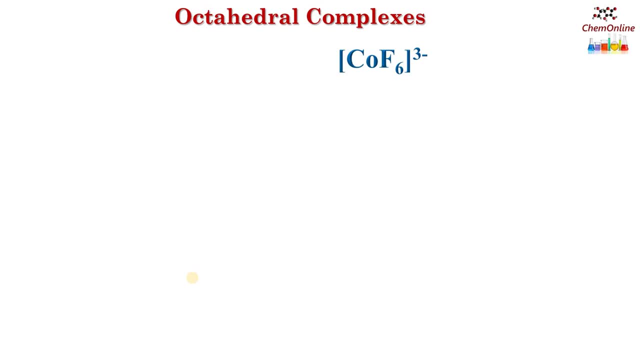 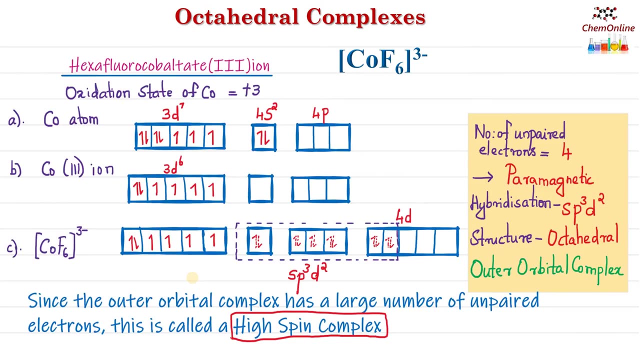 Now let us see some examples of octahedral complexes. First is CuF6 3 minus. So here we have CuF6 3 minus. So first find out the oxidation state of cobalt, which is plus 3.. 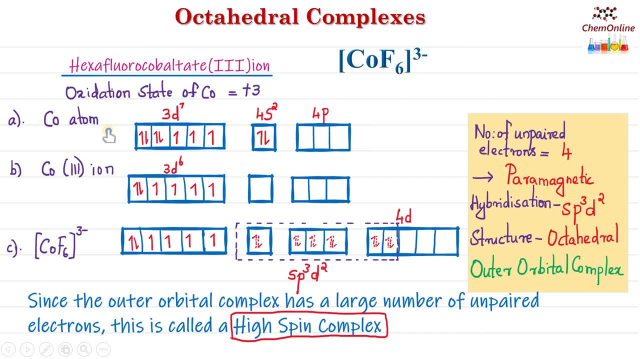 And here you can see that if you look at the ages of cobalt, the cobalt atoms are �o, sg and d. Cobalt atom is a d7 species, So you can write the electronic configuration of cobalt atom. 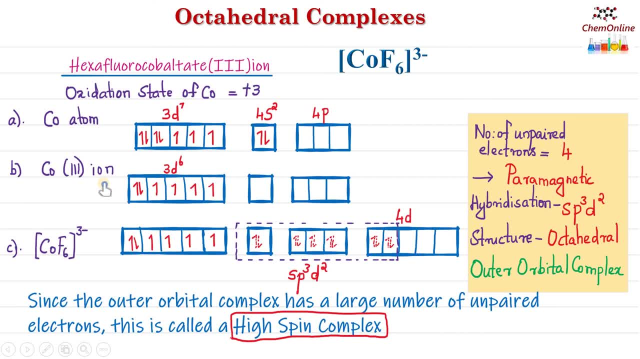 So 3d7, 4s2.. In cobalt, 3 plus 2 electrons from the 4s and 1 electron from the 3d is lost, So the configuration becomes d3.. So that is the configuration for the cobalt atom. 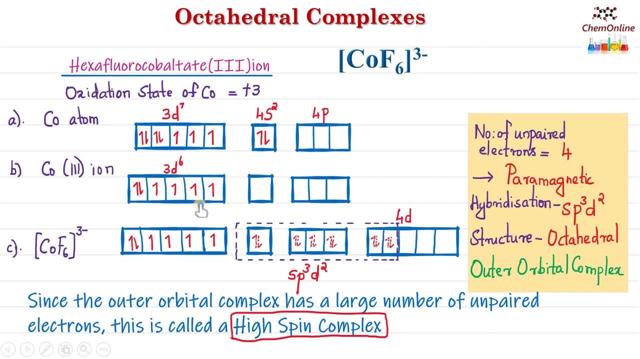 So you can write the electron configuration of cobalt atom: 3d7, 4s2.. 3d6, 4s0, which is shown here. Now, when the 6 fluoride ligands approaches the cobalt, what happens? fluoride is a comparatively weak ligand. All the halide ligands are all weak ligands. 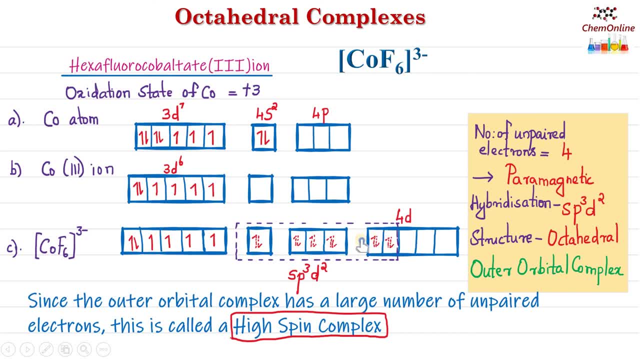 So they occupy the available empty orbitals. So 6 fluoride ions will occupy 1, 4s, 3, 4p and 2, 4d orbitals which are sp3, d2, hybridized and the structure will be octahedral Here the d orbitals. 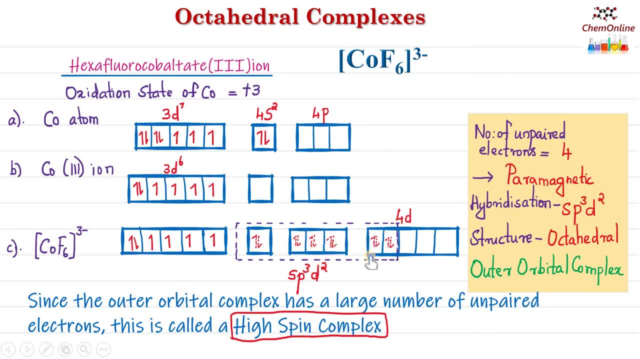 involved in the hybridization is the 4d orbitals, which are called outer d orbitals And hence such a complex is known as outer orbital complex. In Cu F6 3- you can see that there are 4 unpaired electrons. Since it has high number of unpaired electrons, this kind of complex 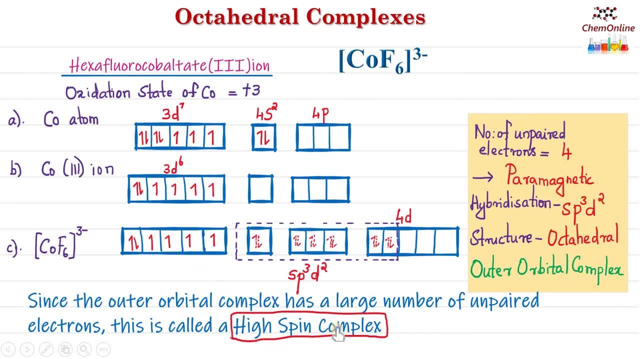 is also known as high spin complex, and obviously this will be a paramagnetic species. So in Cu F6 3- fluoride ion B6- 3- is a paramagnetic species. So in Cu F6 3- fluoride ion B6 3- is a paramagnetic. 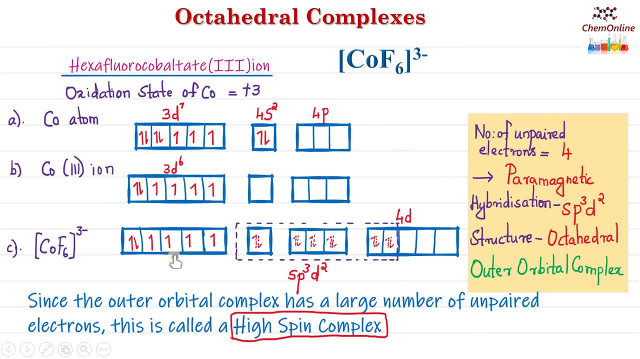 species. So in Cu F6, 3- is a paramagnetic species. So in Cu F6, 3- is a paramagnetic species. So this being a weak field ligands will not cause any pairing up of the electrons and it occupies the available empty orbitals involving 1, 4s, 3, 4p and 2: 4d. the hybridization is sp3, d2 and. 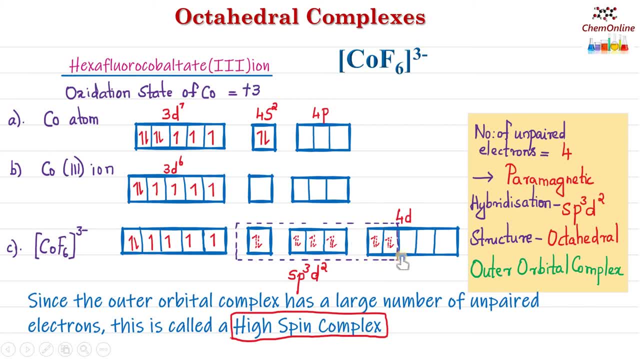 the structure is octahedral. Since the outer d orbitals are involved in hybridization, this complex is known as outer orbital complex. So this is a paramagnetic species. So in Cu F6 3- there are higher number of unpaired electrons, which are sp3, d2, and the structure is octahedral. 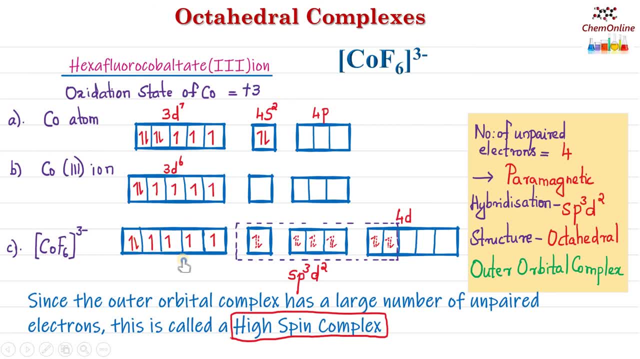 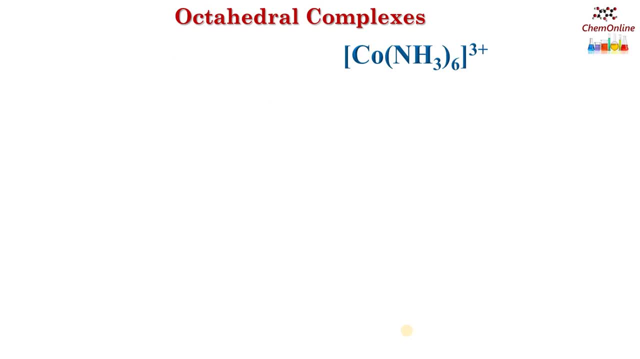 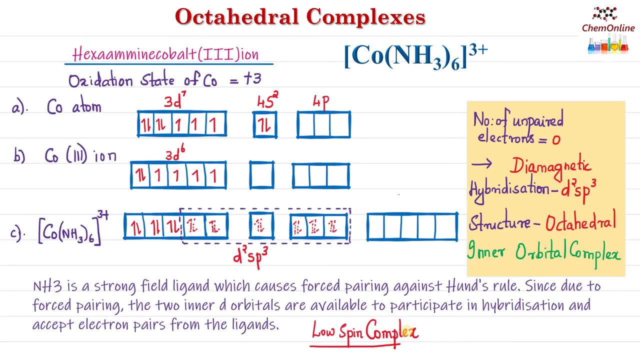 There are large number of unpaired electrons, which are sp3, d2 and the structure is octahedral paired electrons. The species is paramagnetic and such a complex is also known as a high spin complex. The next is another complex of cobalt: Cu, NH3, 6, 3 plus hexamine cobalt 3 ion. 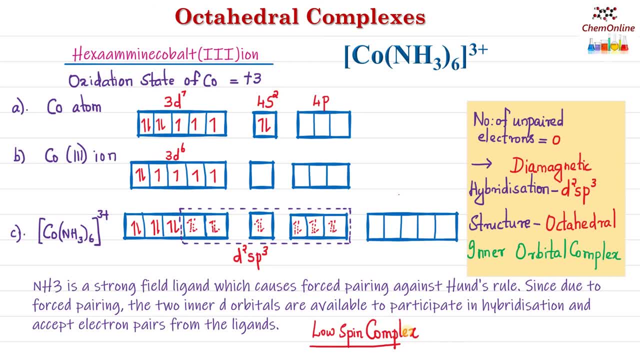 In this complex also, the oxidation state of cobalt is 3 plus So first write the configuration of cobalt atom and then cobalt 3 plus So that is 3D6- 4S0.. Now ammonia is a strong field ligand. 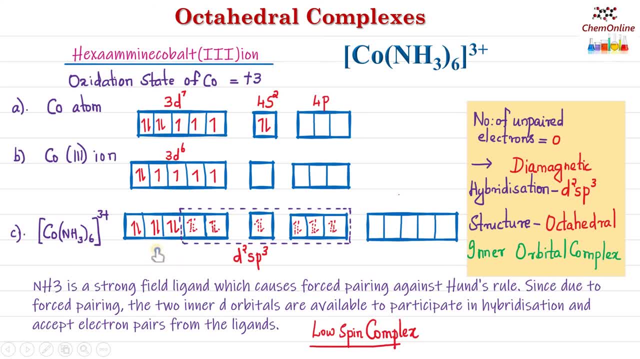 So when they approach the cobalt ion, cobalt 3 plus ion, they will cause forced pairing of electrons in the 3D orbital, which is against the Hans rule. So these two electrons here will get paired up with these two electrons. As you can see here, that means there will be two inner D orbitals available for participating in. 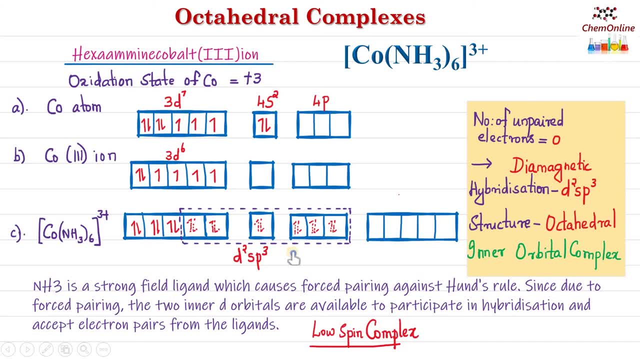 hybridization and they can accept the electron pairs from the ammonia ligand. These dotted arrows represents the electron pairs donated from the ammonia ligand. So you will have two 3D orbitals: 1, 4S and 3D3.. 3, 4p orbitals, making the hybridization d2sp3, and the structure will be again octahedral. 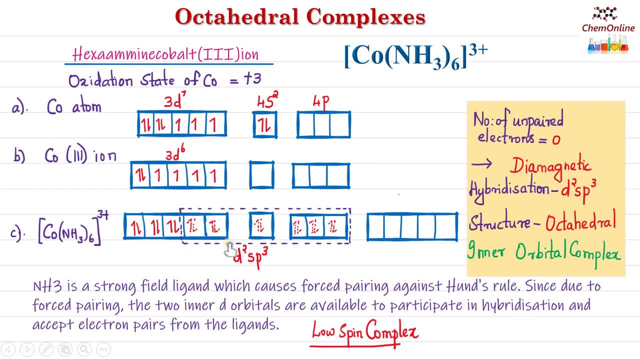 And here, since the 3d orbitals or the inner orbitals are involved in hybridization, this complex is known as an inner orbital complex. In the previous case it was the 4d orbitals, which is an outer orbital. Here the inner 3d orbitals are involved and hence it is also known. 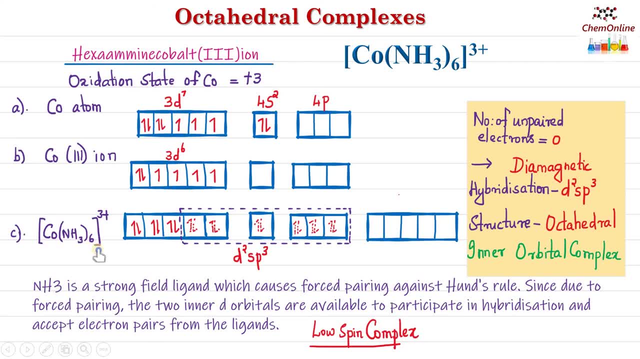 as inner orbital complex. Also, in CO NH363+ all the electrons are paired up. That means the species is diamagnetic. So since all the electrons are paired up, there is no knit spin. So such a complex is also known as low spin complex. 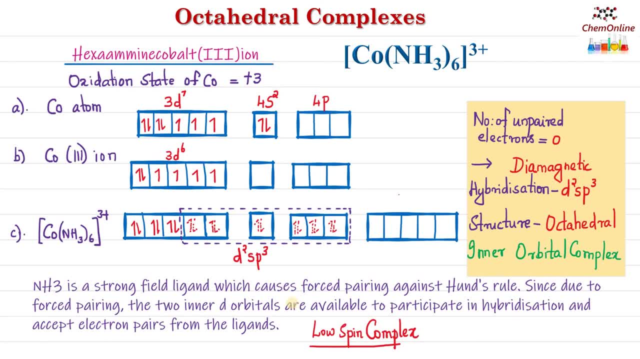 So in CO NH363+. Ammonia is a strong field ligand which cause forced pairing of electrons in the metal d orbitals. So the inner d orbitals become vacant and can involve in the hybridization. So the hybridization becomes d2, sp3 and the complex formed is known as inner orbital complex. 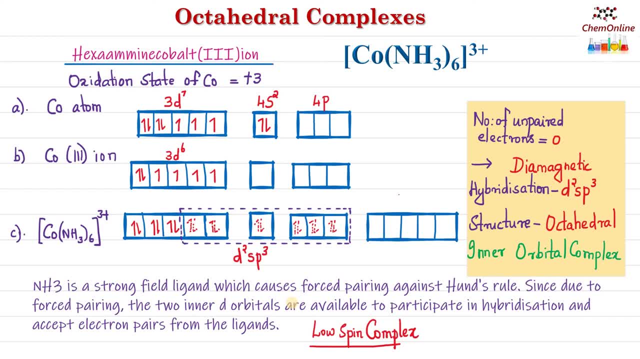 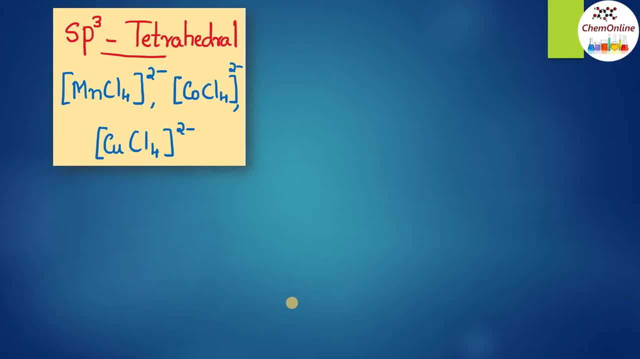 All the electrons are paired up here, So the complex is diamagnetic and it is also a low spin complex. Now let us see some other examples with different hybridization and geometries. With sp3 hybridization the structure will be tetrahedral. 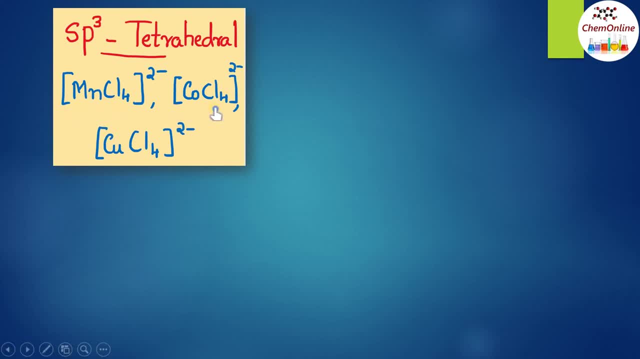 Other examples include MnCl4 2-, CoCl4 2-, CuCl4 2-, etc. And if it is dsp2, the structure will be square planar: CuNH3, 4-2+, PtNH3, 4-2+, etc. 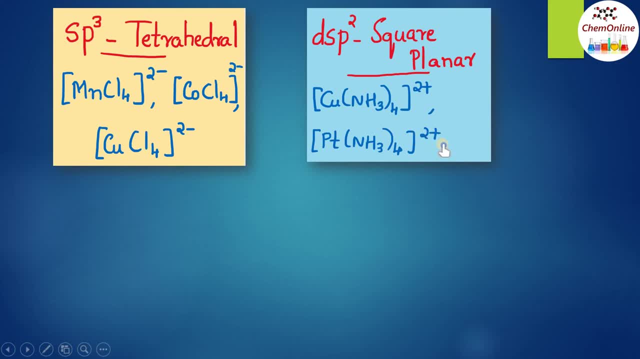 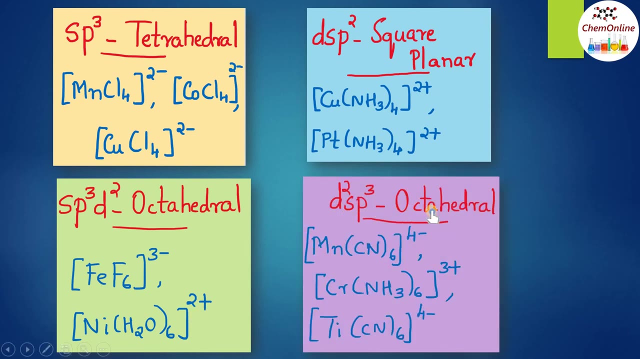 Form square planar complex. Now with sp3 d2 forming octahedral complex like FeF6, 3-, NiH2O6, 2+, etc. d2 sp3 also forms octahedral complexes. Examples include MnCn6, 4-, CrNH3, 6-3+, TiCn6, 4-, etc. 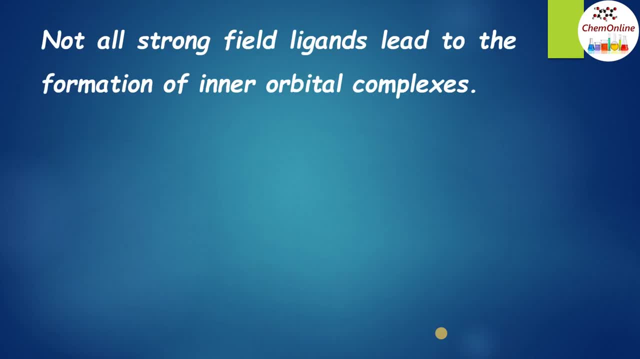 We have seen that Strong field ligands usually causes pairing up of the electrons and resulting inner orbital complexes, Whereas weak field ligands usually form outer orbital complexes. But this is not always the case. Not all strong field ligands lead to the formation of inner orbital complexes. 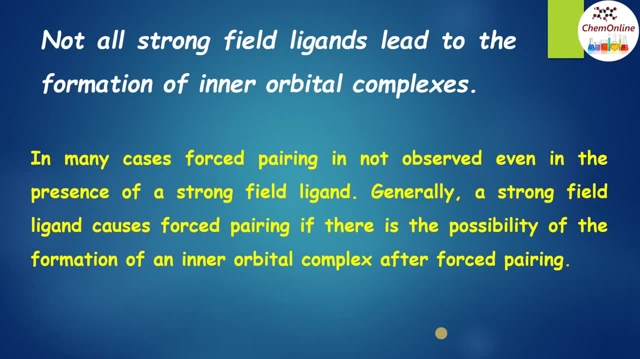 In many cases it was observed that even in the presence of a strong field ligand the force to pairing does not, And generally a strong field ligand causes forced pairing only if there is a possibility of the formation of an inner orbital complex after forced pairing. 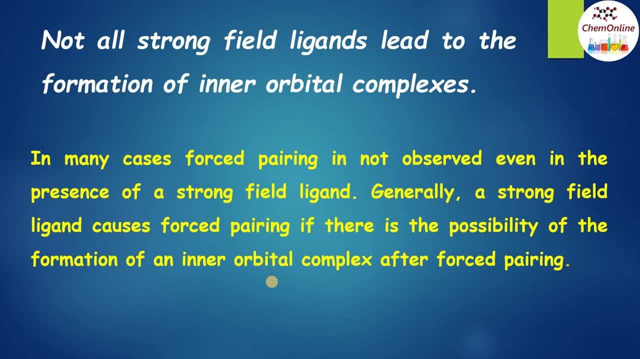 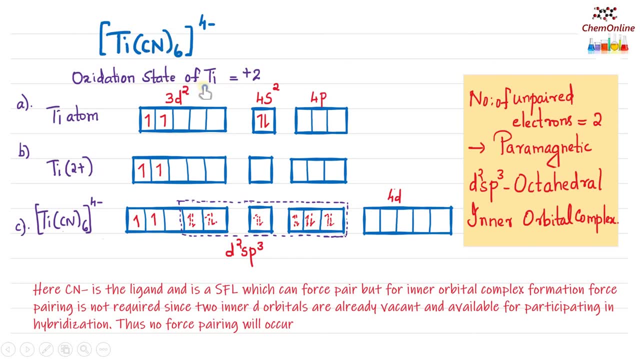 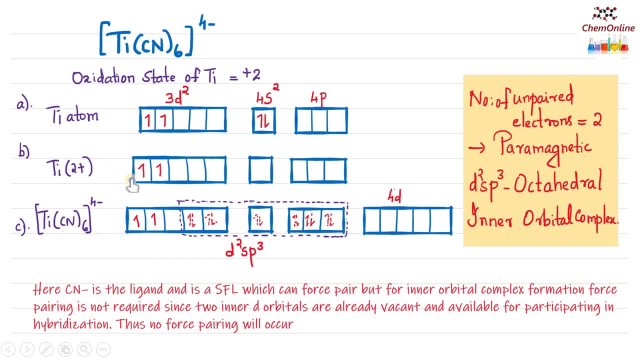 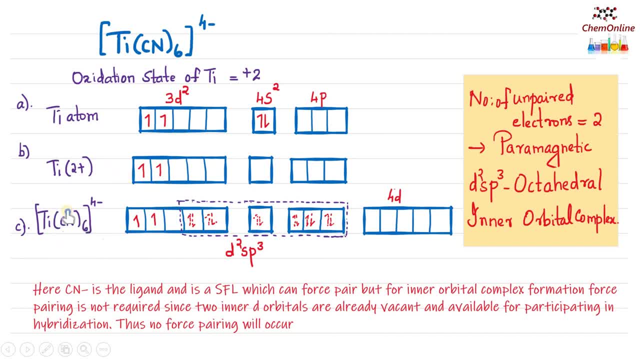 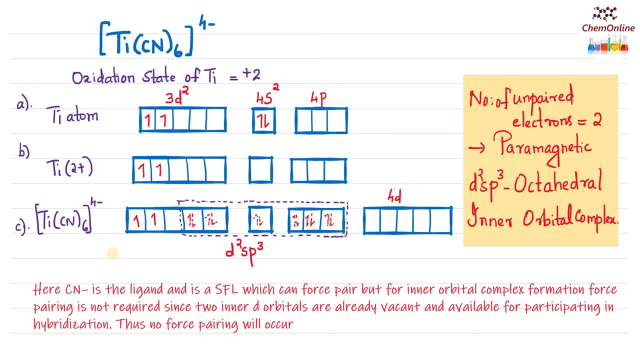 which causes pairing up of the metal d electrons. But here there are inner d orbitals which are vacant and available for hybridization. That means there is no need of pairing up of the electrons, So no forced pairing will occur, While the electrons from the cyanide ions will occupy the two inner d orbitals 1- 4s. 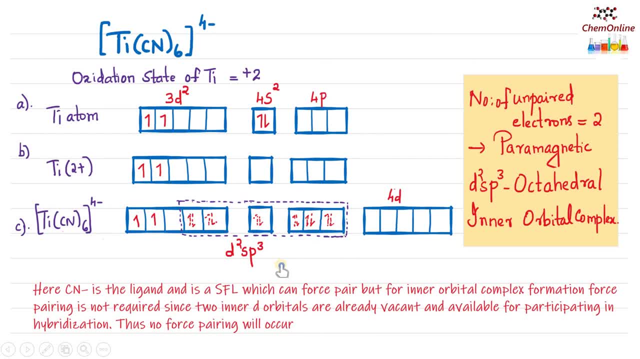 and 3, 4p, involving d2, sp3 hybridization, and the structure will be octahedral And since there are two unpaired electrons, the complex is paramagnetic. So here, although cyanide is a strong ligand, there is no forced pairing because the inner 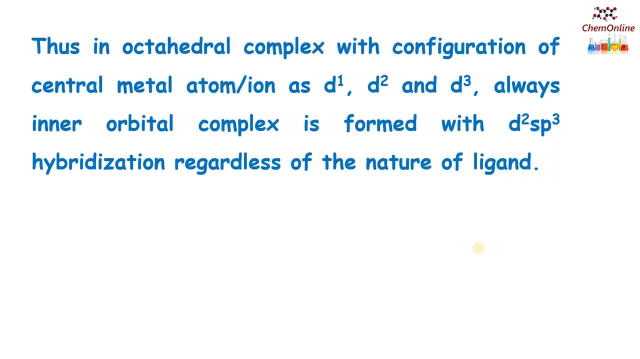 orbitals are already available. So generally we can say that In octahedral there is no forced pairing. So generally we can say that Here also there is aρ complex with the configuration of the central metal atom ion as d1, d2, d3. 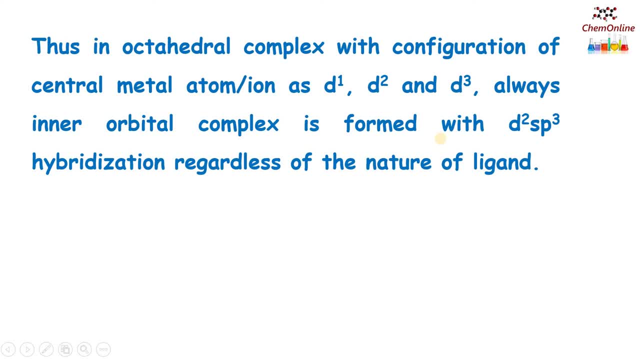 always inner orbital complexes, preferably formed with d2- sp3 hybridization, regardless of the nature of the ligand, that is, whether it is a strong field ligand or weak field ligand, always an inner orbital complexes formed with configurations of d1, d2 and d3. 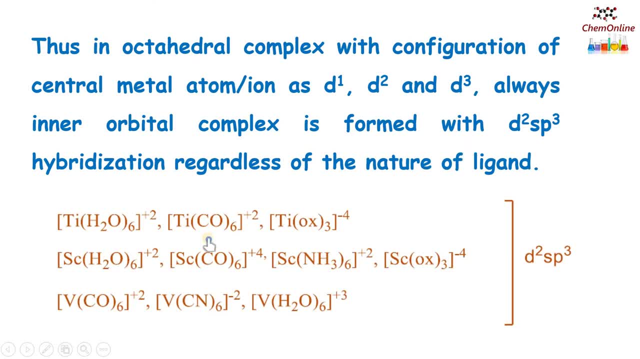 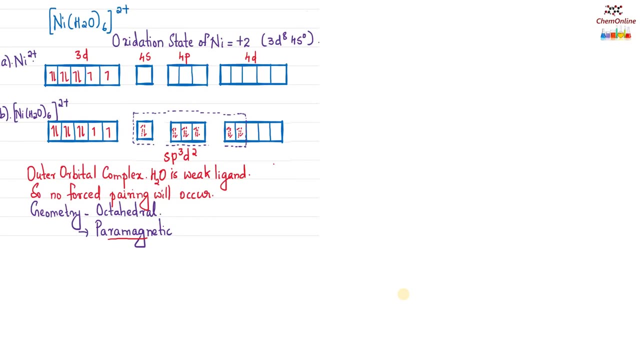 Here we can say that. So, dear viewers, coordination complexes involving d2sp3 hybridization with both strong field and weak field ligands. Now consider an example of nickel complex: NiH2O6 2+. Here the oxidation state of nickel is 2+. 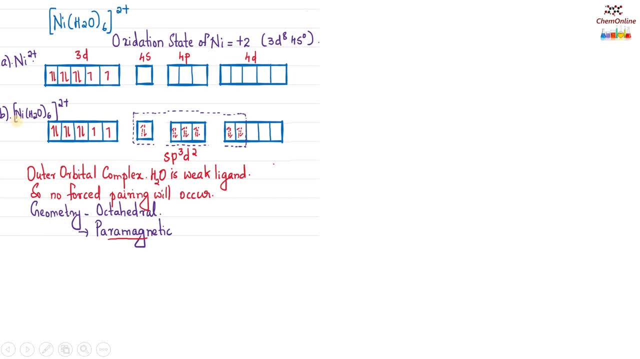 is 3d8, 4s, 0.. Now in NiH2O6 2+, H2O is a weak field ligand, So no forced pairing of the electrons. so the electrons from the H2O will occupy the available orbitals. So that is 1, 4s, 3, 4p and 2, 4d. 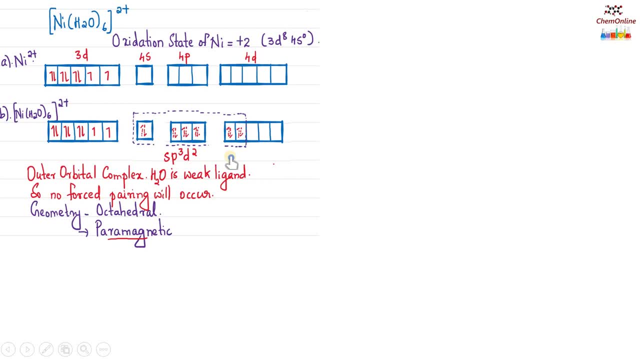 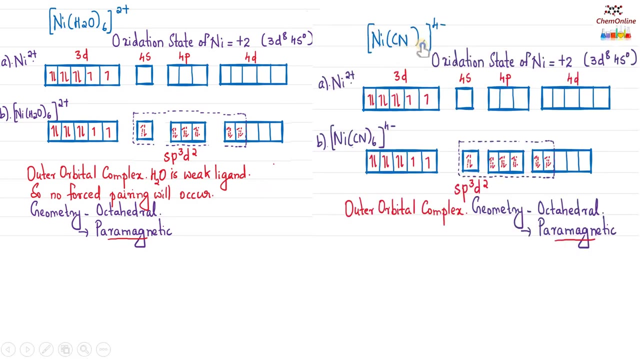 forming sp3- d2 hybridization. The structure is octahedral and since there are unpaired electrons, the complex is paramagnetic, and this is an outer orbital complex. Now consider the nickel complex containing six cyanide ions, NiCn6 4-. 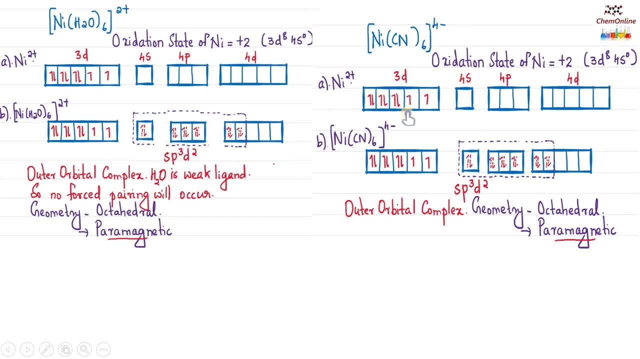 Here also, the oxidation state of nickel is 2+, so the nickel 2- plus ion was 3 d 8 configuration. Now we know that the cyanide ions are strong field ligands, so we expect a forced pairing of electrons in the three d orbitals. But actually no forced pairing of electrons will occur. 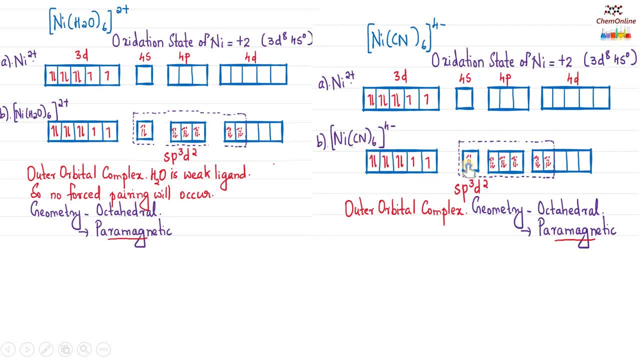 but instead the electrons from the cyanide ions occupy the available vacant orbitals, that is, 1, 4, unspecified- 4, d8.. 4s, 3, 4p and 2, 4d. Again, sp3, d2, hybridization with octahedral geometry, and this is also an. 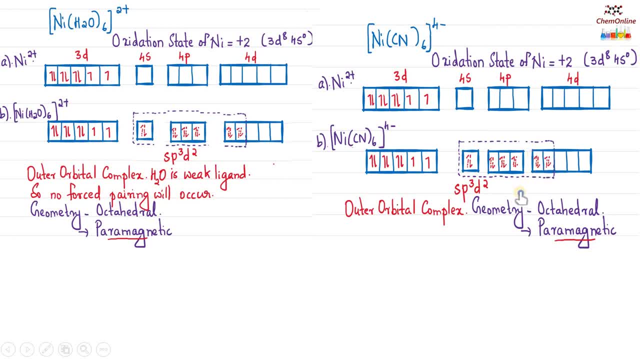 outer orbital complex because the 2, 4d orbitals are involved. Here you can see that though cyanide is a strong field ligand, there is no forced pairing of the electrons because even after forced pairing only one inner d orbital will be available, And we know that for the formation of 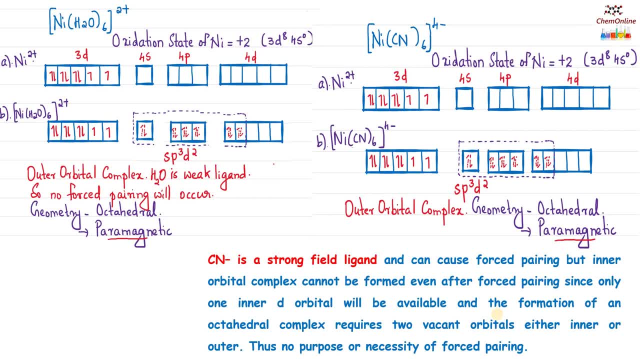 an octahedral complex, we require two vacant, either inner or outer d orbitals. But here, after pairing, there will be only one vacant d orbital, So there is no necessity of forced pairing. Instead, the electrons from the cyanide ions occupy the other available orbital. 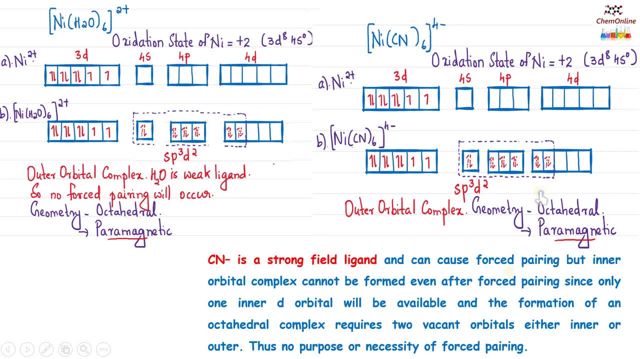 That is an outer orbital complex, And here also there are two unpaired electrons, So the species is paramagnetic. So in these two complexes of nickel, H2O is a weak field ligand, while cyanide is a strong field ligand, But in both these cases the hybridization is the same. 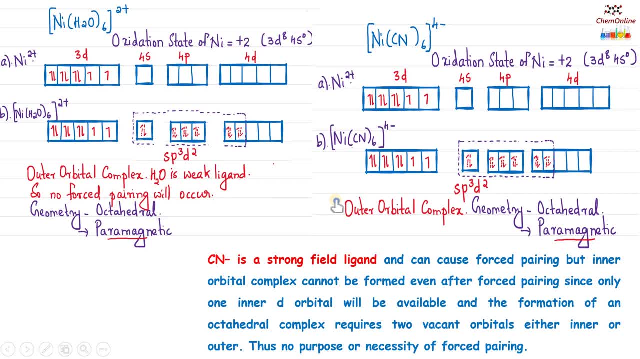 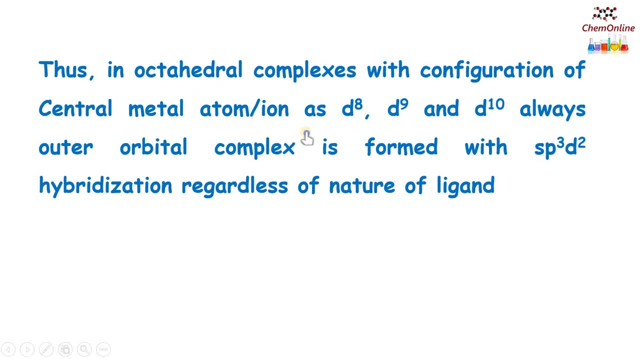 sp3, d2. Both these complexes form outer orbital complex. So we can generalize that in octahedral geometry we have an outer orbital complex. So we can generalize that in octahedral complexes with configuration of the central metal atom or ion as d8, d9 and d10, always. 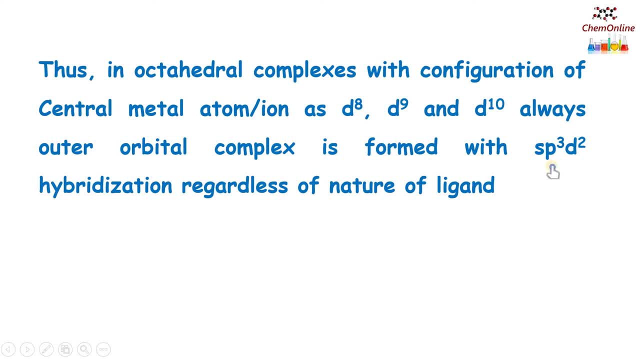 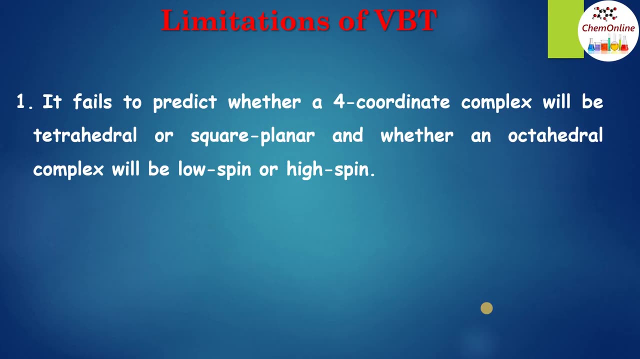 preferably form outer orbital complex with sp3- d2 hybridization, regardless of the nature of the ligand. These are some examples of outer orbital complexes. Now let us move on to the limitations of valence bond theory. Valence bond theory could successfully form an outer orbital complex, So we can generalize that in octahedral geometry. with sp3- d2 hybridization, regardless of the nature of the ligand. These are some examples of outer orbital complexes with configuration of the central metal atom or ion as d8, d9 and d10 always preferably form an outer orbital complex with configuration of the central metal atom or ion as 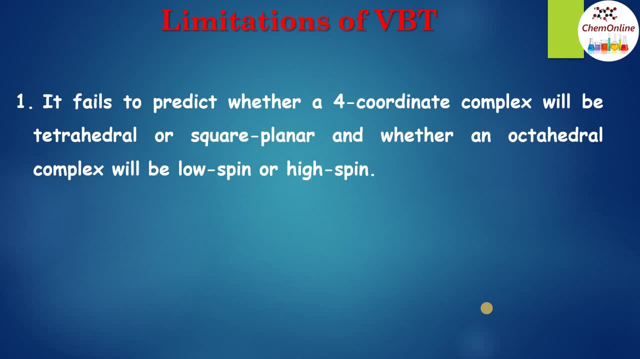 sp3, d2 hybridization, regardless of the nature of the ligand. These are some examples of the magnetic properties as well as the geometries based on hybridization, But it fails to predict whether a four-coordinate complex will be tetrahedral or square planar, and whether an 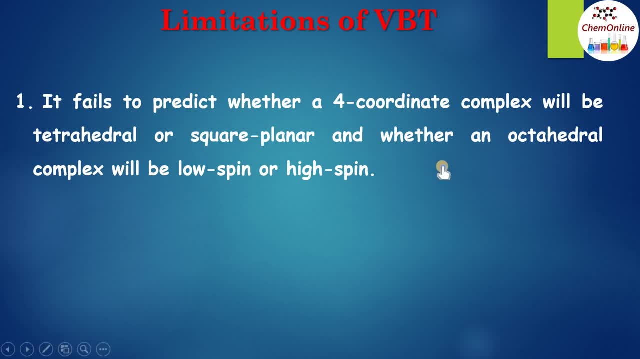 octahedral complex will be low spin or high spin. That is what factors compel the metal ions to utilize the d orbitals of different principal shells, That is, of the inner orbital of the metal ion or outer orbitals, is not explained by the valence bond theory. It fails to distinguish.